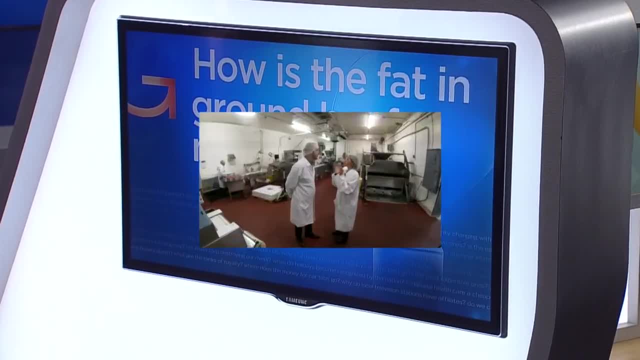 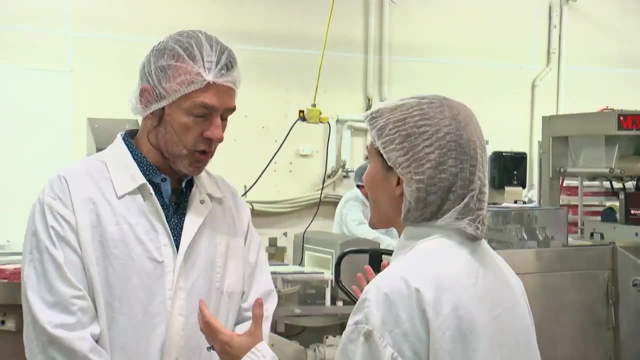 before social distancing guidelines were in place. So tell me where we are. We're at Swanson Meat Company in South Minneapolis. You provide meat for restaurants all over the Twin Cities. All over the Twin Cities, some of the most famous burger places. 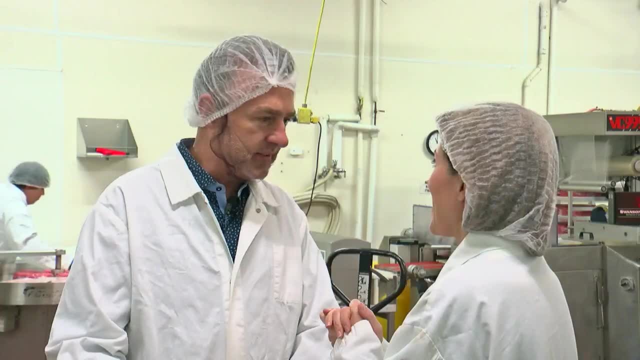 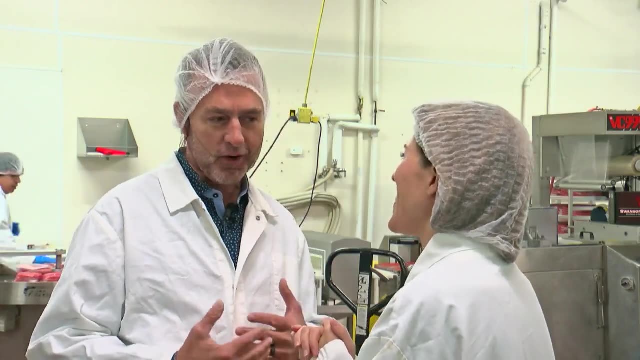 from Matt's to Lion's Tap to 50's Grill and St Danette and Lurkot Burgers. We do Revival. Oh my, A lot of burger contests tell who wins the burger, but they never tell where it comes from. 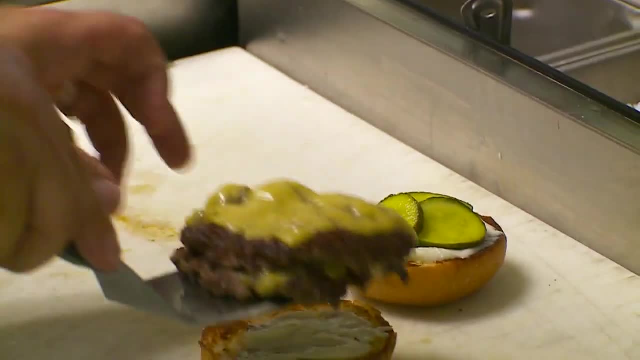 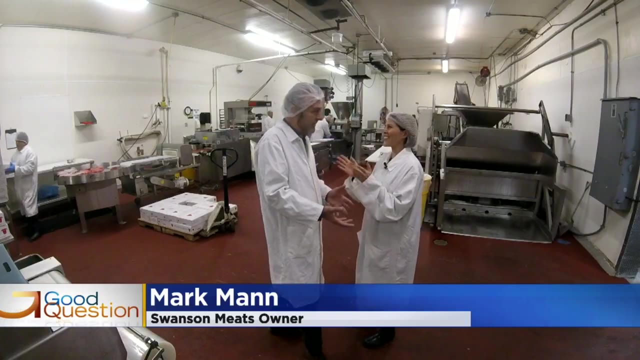 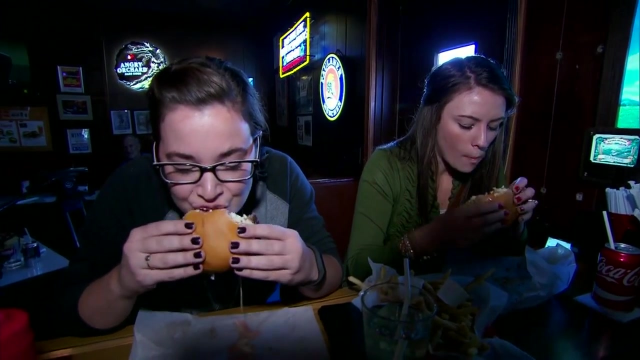 And that's right here, Right? So what is the lean content? when it comes to the fancy stuff, Every restaurant has their own recipe and, due to confidential reasons, we can't tell, But it's somewhere between 75% and 85%, and that's one of the reasons when people go out to restaurants. 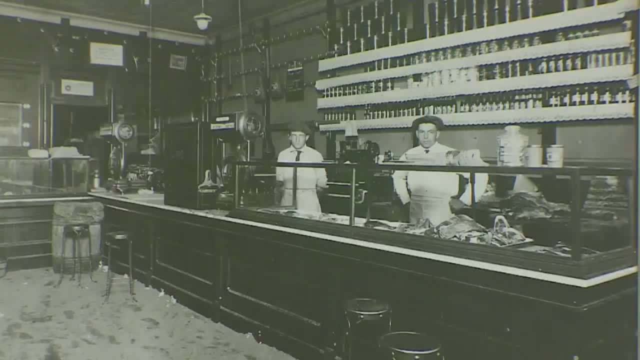 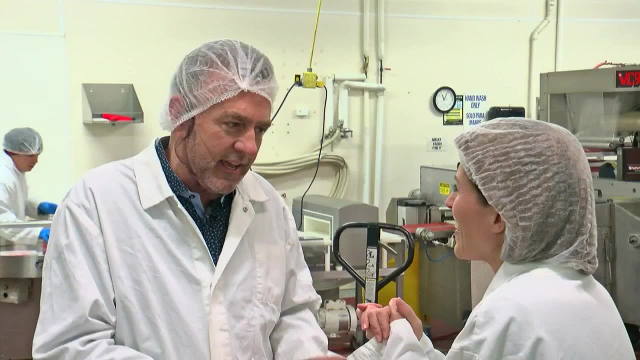 they don't know where to go. Right, They like their burgers better than they do at home. Good point. Decades ago, butchers would measure lean content by sight. It was kind of like the old masters would just look at it and say it's 80%. 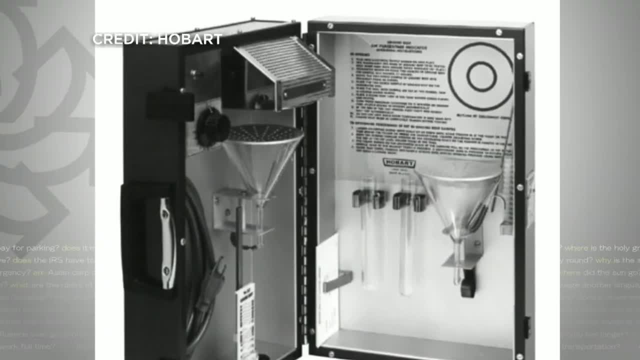 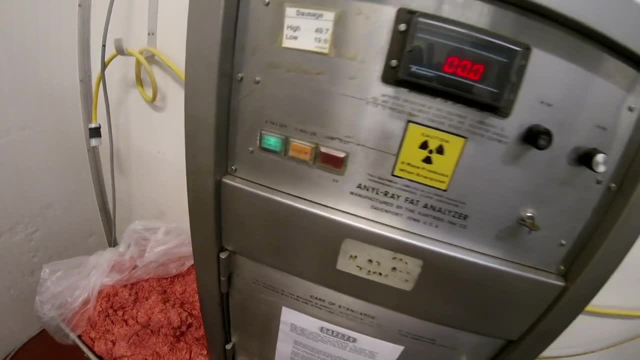 In fact, in the beginning days that's how we did it. Then they got machines with grills and test tubes. We'd take a burger and you'd have to cook it off and measure the drippings. But now Swanson Meats has this $50,000 fat analysis machine. 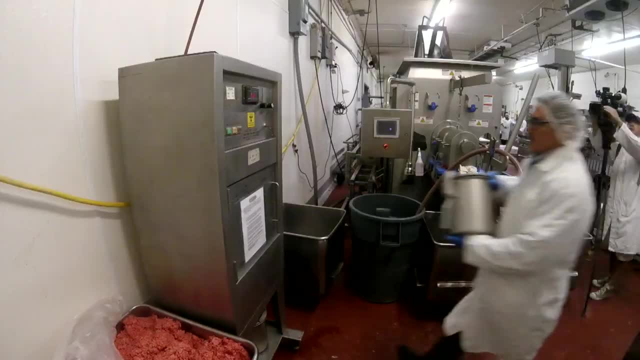 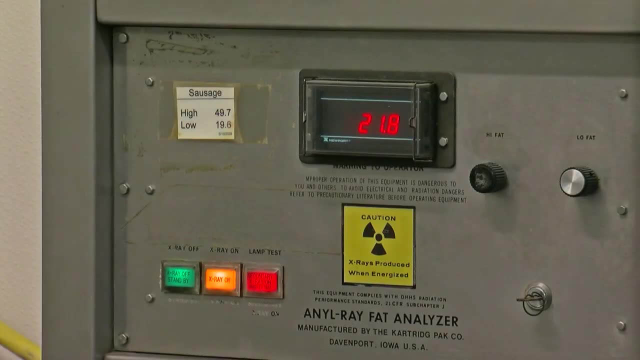 It's actually an X-ray. The ray is a light beam that goes through the beef Beef, which gives us an instant fat content versus lean. It gave us the answer in seconds. Are you always within .1 or .2%? We try to be. 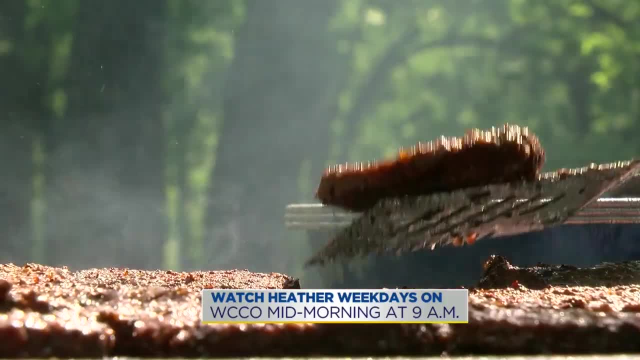 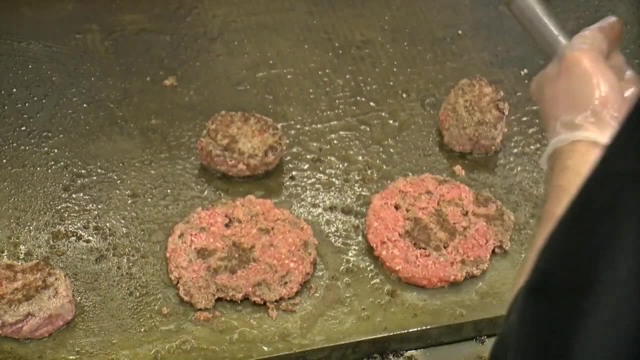 Mann recommends the 80% or 85% lean for your backyard grill. That'll avoid flare-ups, So you would not have a forest fire. And in the mid-70s, when you're eating out, 70% lean is the lowest allowed by law. You're telling us, don't be afraid of the 75%. Don't be afraid of it because your heart doctor wouldn't tell you to do it, Heather Brown, But your taste buds would tell you to do it. WCCO 4 News. 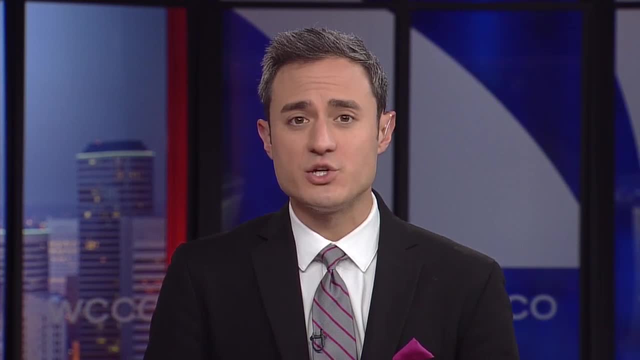 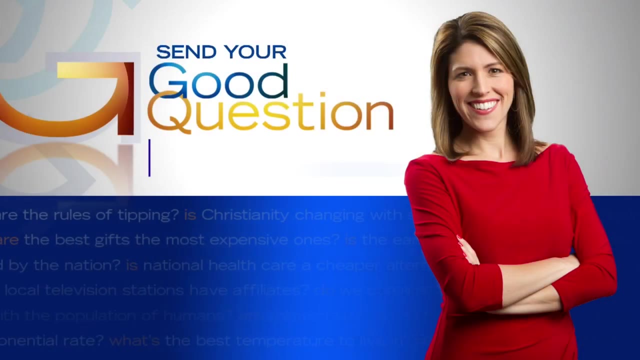 The USDA regulates ground beef labeling. At Swanson Meats a USDA rep on site does daily spot checks. One thing she checks is the lean content of the ground beef. If you have a good question for Heather, email her by visiting WCCOcom. slash links. 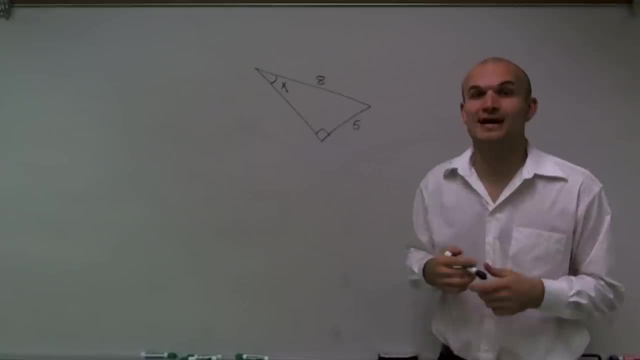 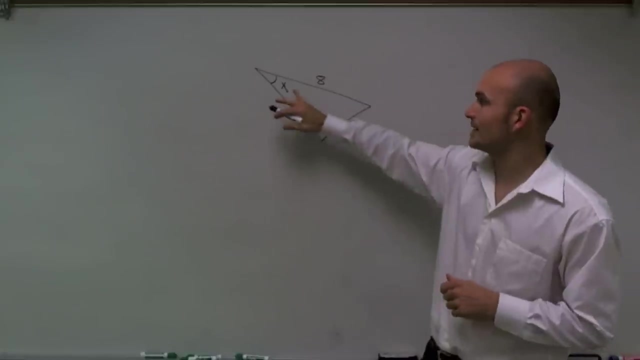 Welcome. What I want to do today is show you how to find the missing measurement of our indicated angle. So what we have here is we have a triangle with I have a missing angle measurement for an angle here which is x, And the important thing to understand about this triangle is I have